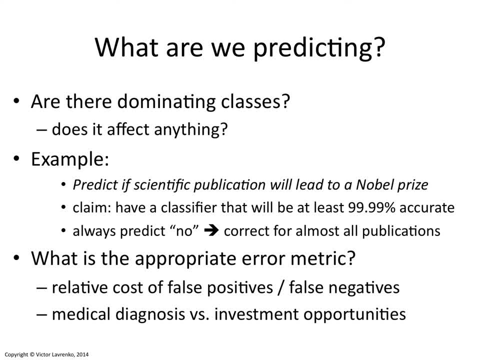 Okay, so that is an example of unbalanced classes. It's an example where one class publications that don't lead to a Nobel Prize are a lot more numerous orders of magnitude bigger than another class. And what do you do in those situations? Basically, you have to ask yourself what is the right error metric. 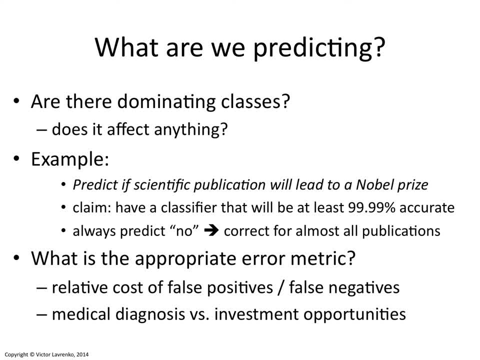 What is the right error metric to use? Usually, what we use, and what we'll be using in most of the course, is classification accuracy. What percent of the training data did our algorithm get correctly? And what you want to do in this case is you want to consider? 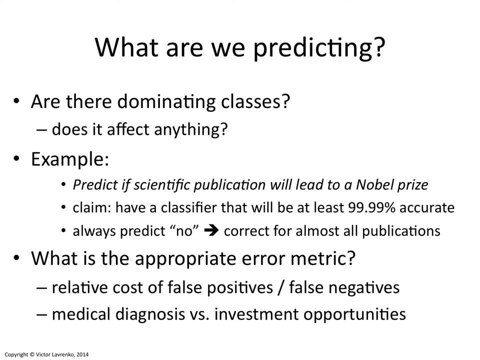 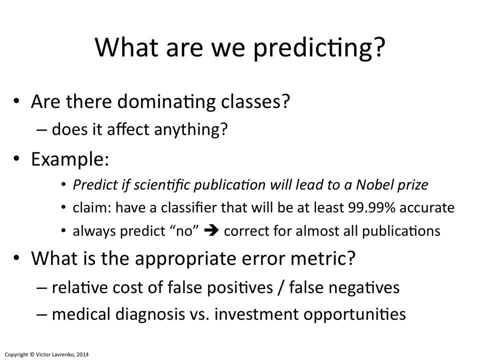 So if you put different weights on those, that is one way to address the problem. Now, if you're not convinced that this is actually a big problem, so you could say: all right, so always saying no is 99.99% accurate. 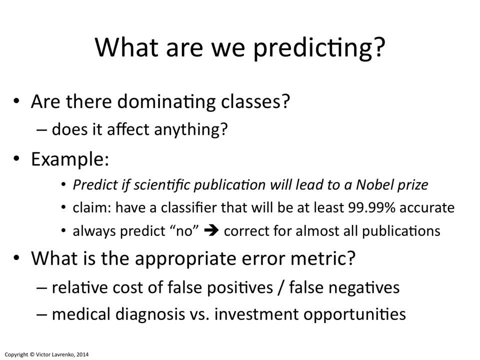 but if I actually got things correctly, it would be 100%. So I just need the right learning algorithm, And unfortunately that's not the case. You could have a very good learning algorithm, and it would still not do the right thing if you give it the wrong metric. 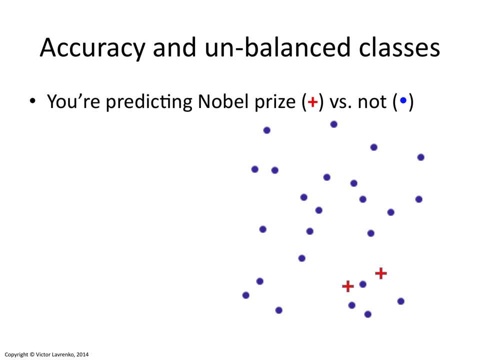 the wrong accuracy measure to optimize. So suppose I have this little scenario. That's my data set. The blue guys, that's all the articles that didn't get the Nobel Prize, And the red pluses, these are the guys that did win the Nobel Prize.